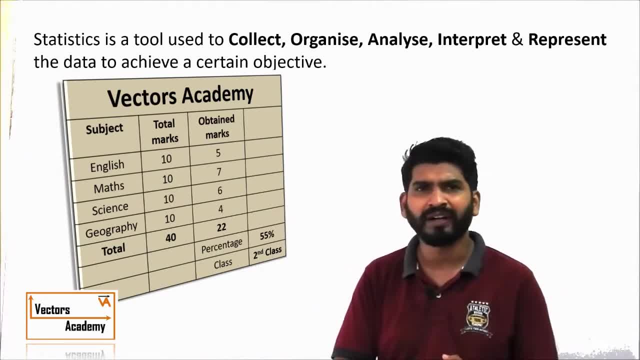 fact is actually used everywhere. You have seen a simple example of report card right. So statistics can be used in medical field to understand the growth of certain culture of bacteria. It can be used in business field to understand what is the relation between the price and the sales. It is. 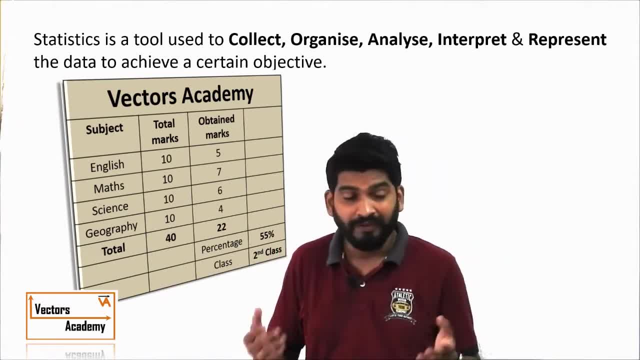 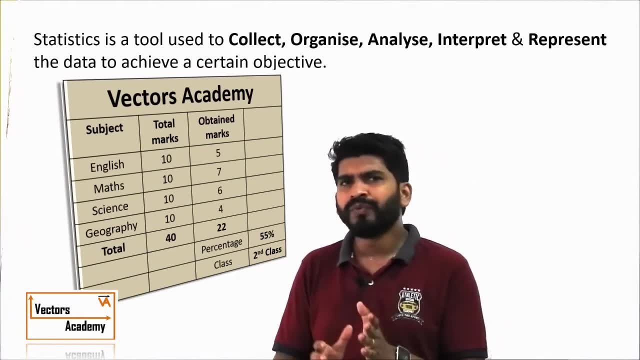 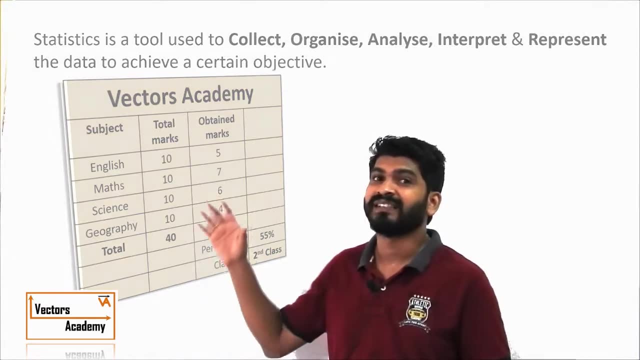 used in the engineering field. It is used everywhere, almost everywhere, In fact. wherever you play with something, you are using statistics. Now, before moving on to the advanced level of statistics, one should first know the basic principles of statistics. That is, the central tendencies Now. 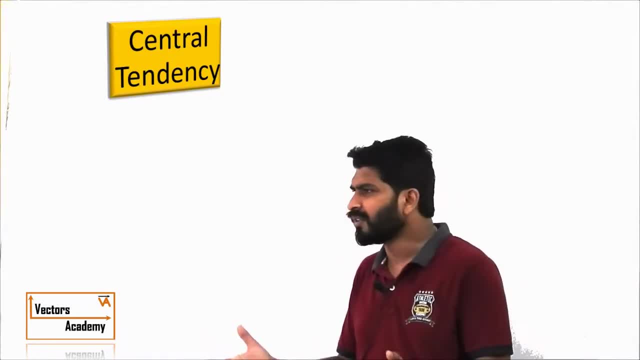 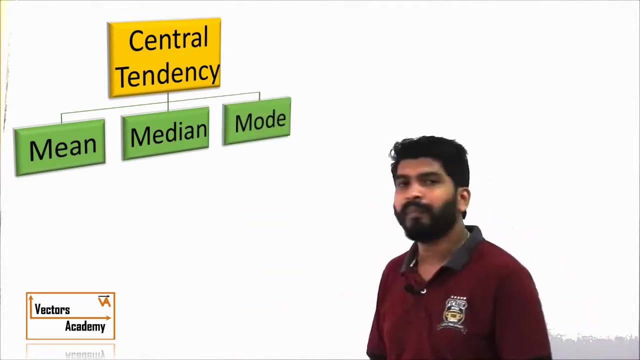 what is the central tendency? Now, the central tendency can be termed as a single element where all the collected data converges. Now, again, to understand this better, we will divide central tendency into its main main components, That is, mean, median and board. Now, mean, Many of you are aware of what is mean. That is the average Median. Median is the 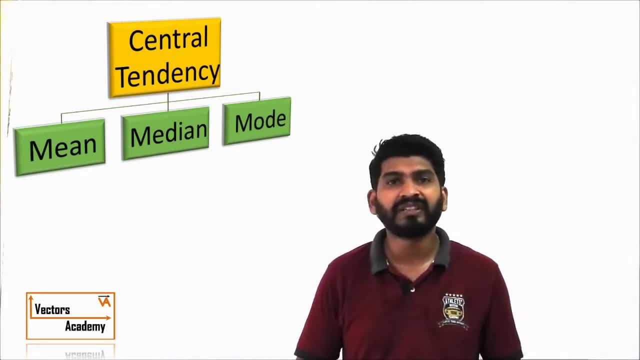 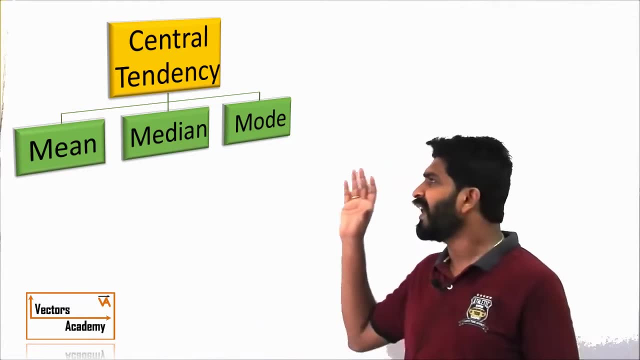 center most value of the given data And mode. Mode is the data which which occurs maximum number of times in the given observation. Now let us take a quick example to understand where these mean mean, how to calculate these mean- median and mode- and where they are actually used. 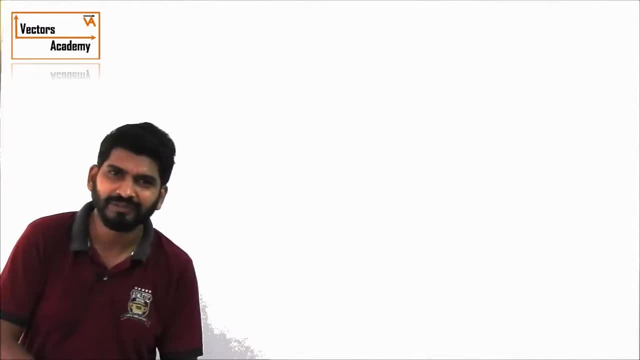 Now consider a teacher with a class of around 10 students. Okay, we will take a smaller number, 10, for now. Now this teacher takes a test of all the students, Takes a max test of all the students, And these are the marks which. 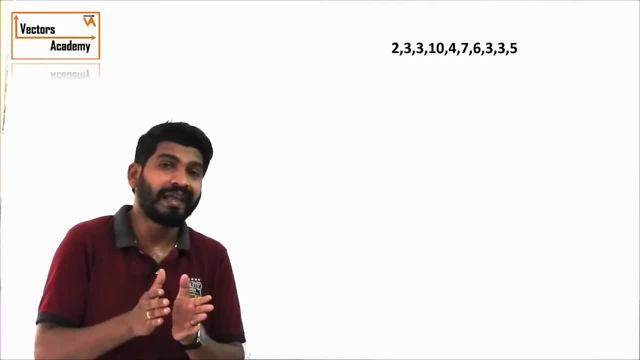 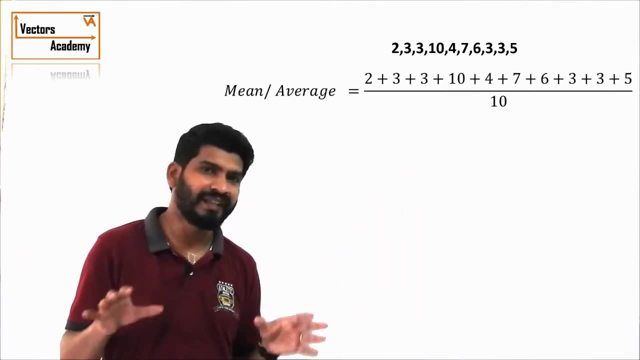 the students get Okay. now how do we calculate the mean? Mean is the average, And many of you are aware of how to calculate the average. We just add all the numbers and once you are done adding all the numbers, we divide by total number of students. Okay, so that comes out to be 4.6.. That is the 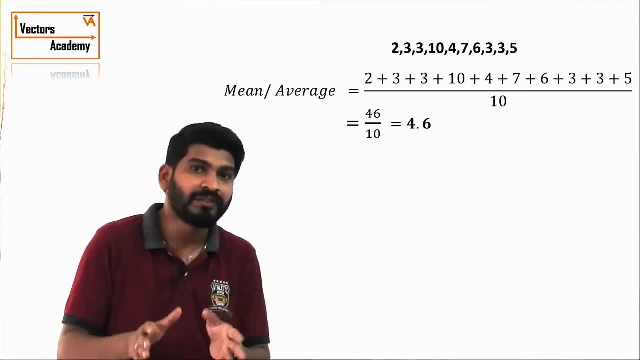 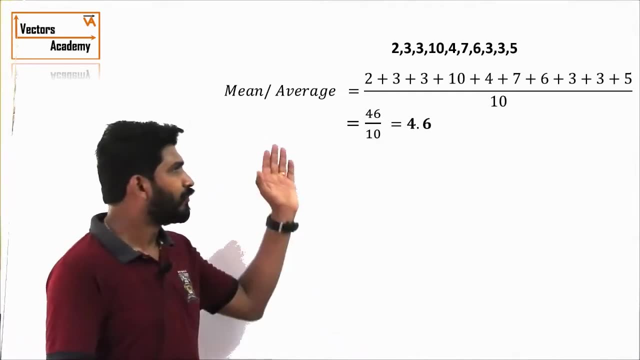 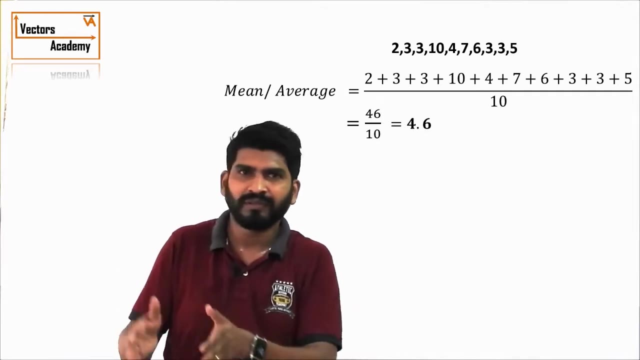 mean. So I can say the average intelligence of a person or of a student in that classroom for maths is less than 4.6 out of 10.. Okay now, What if our aim is to divide the class in two divisions, One containing good students in a, Maths and another not so good students in manufacturers? Okay, so for. 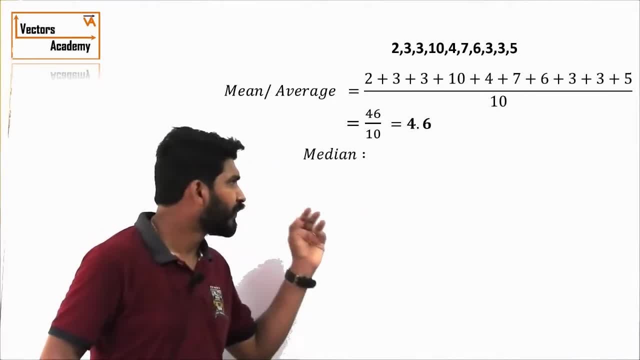 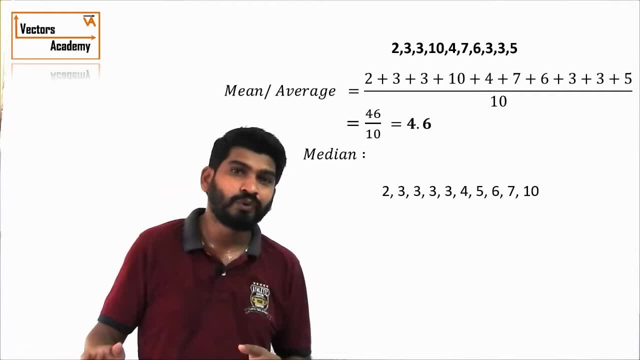 that we cannot use the mean. Now what happens if you use mean? Now? look at this data. We have organised the same data in the ascending order And if I say the students getting less than for 6, the average marks Less than four point six in one class, greater than full point six in the 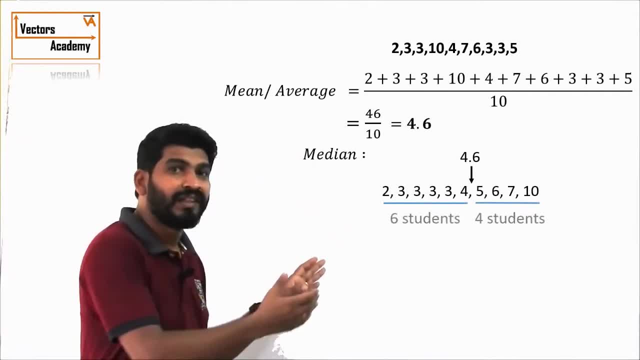 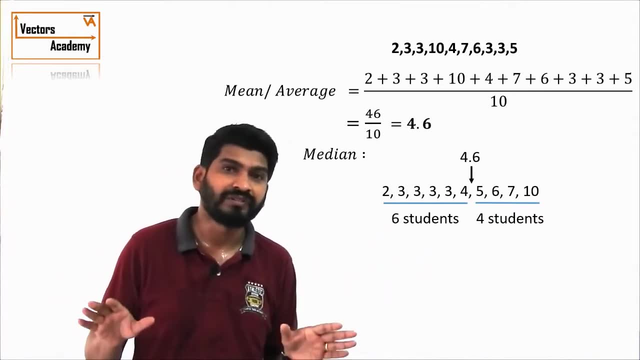 other class. That will not do, because if we divide in such a way, the one class will contain 6 students and the other will contain 4 students. So they are not equal classes, not equal divisions. For that median is used. Now what exactly is median Once we organize them in the 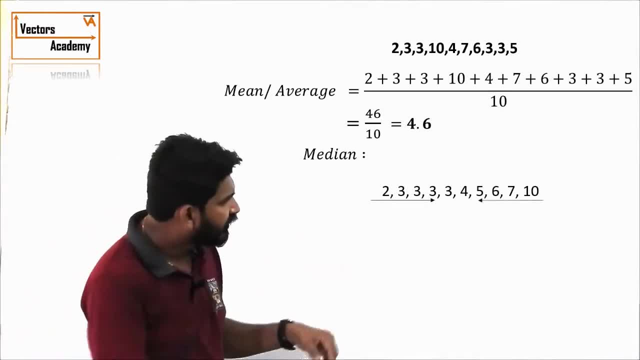 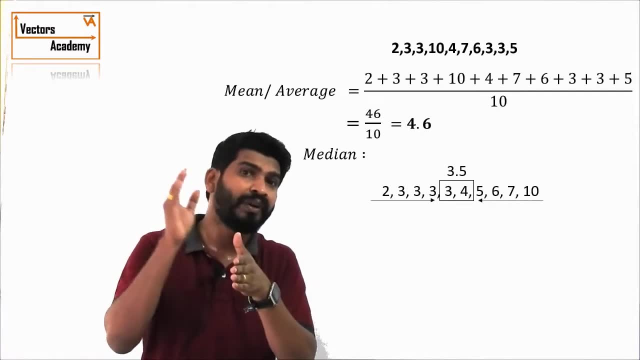 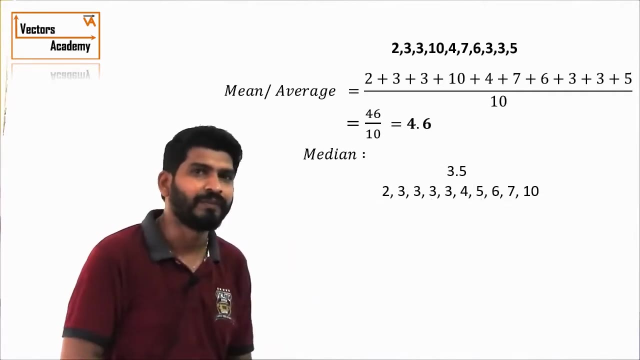 ascending order. you can see if you start approaching from both the sides. there are two numbers, 3 and 4, which lie in between, So that 3 and 4, the number which lies between 3 and 4, that is 3.5.. 3.5 is called as a median. So what is a median? Median is the centermost value. 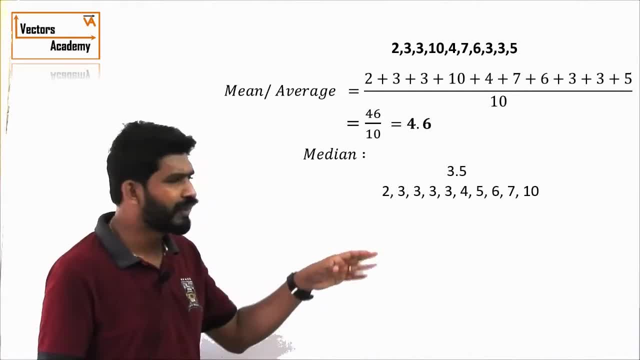 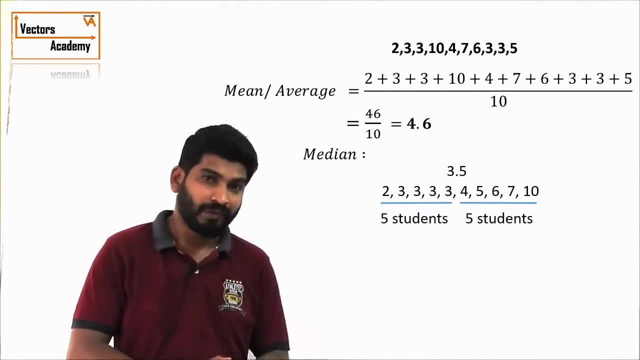 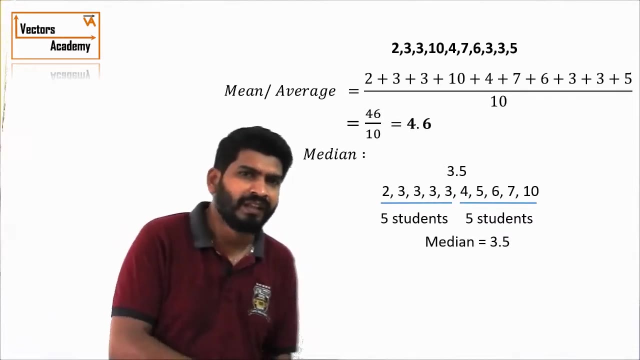 Now we can say: the students getting less marks than 3.5 in one division and more than 3.5 in another division. Now we have two equal divisions of the class. So median actually gives you the centermost value which can be used to divide the data into equal halves. Now, once you get mean, 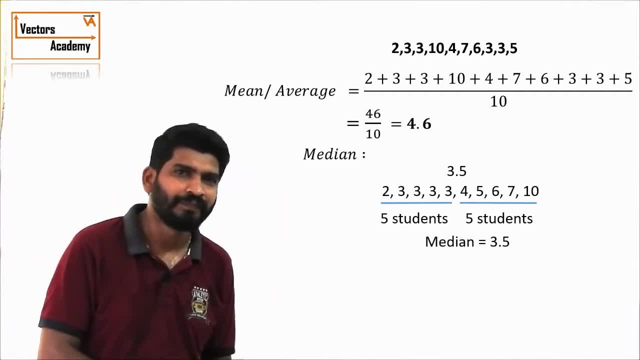 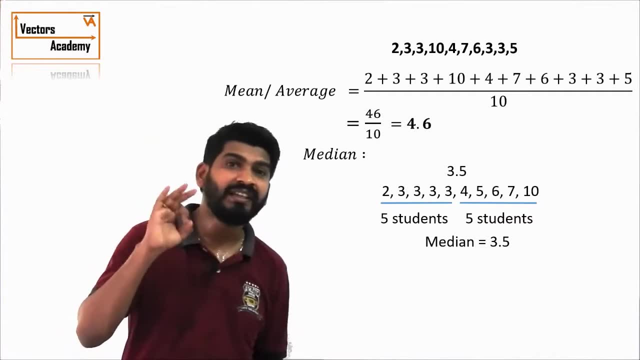 and median. why is mode used And what is exactly mode? Mode is the value which occurs maximum number of times. You can see in the given data 3.. 3 are the marks which occurs maximum number of times, So hence 3 can be. 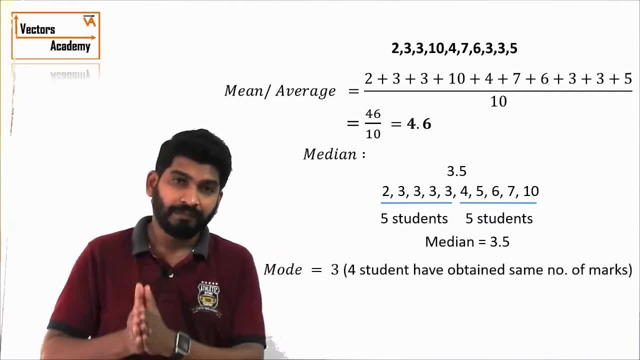 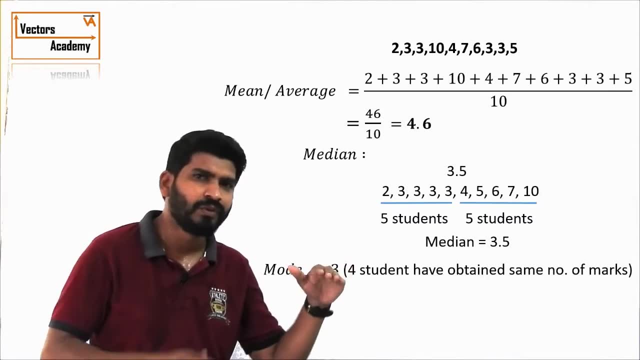 termed as mode, Now why it is used. Now suppose we need to have a research done on these students. but the students should be of the same intellectual level, not varying intellectual level. So suppose if I select a student getting 10 marks and one who gets 2 marks, 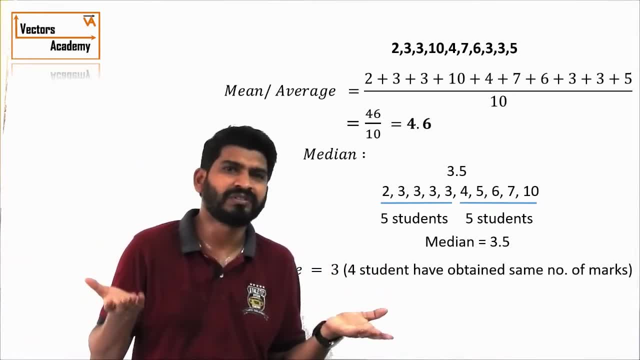 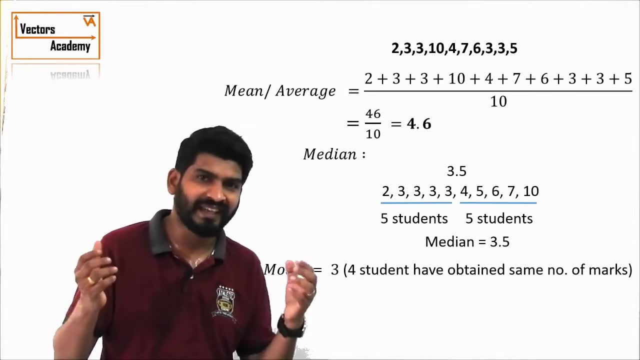 conducting a test on these students won't serve my purpose, because I know the intellectual level is quite different. For that I need maximum number of students which I can get of the same intellectual level and that can be obtained by mode. So there are four students who have.